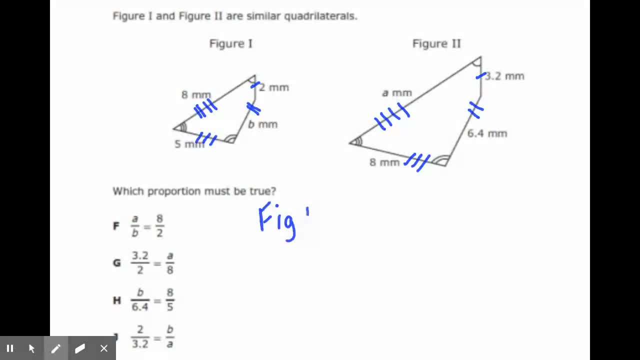 being consistent, All right. so if they put figure one on top on the left, then figure one must also be on the top on the right-hand side. All right, they can't do figure one over figure two on the left and then flip it and do figure two over figure one on the right. That. 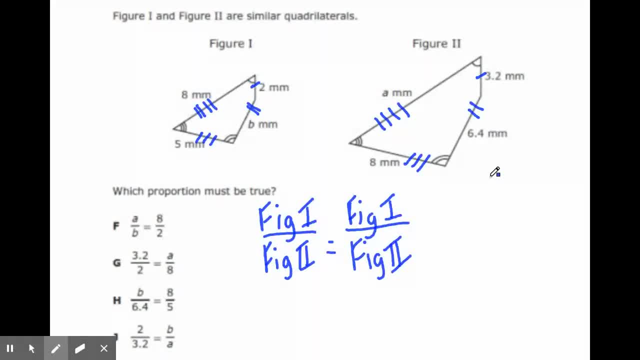 would not work for our proportion. So let's go ahead and look. Our first one says A over B, So this one is saying that A is corresponding to B. Looking at our congruency marks, though, we can see that A has four. 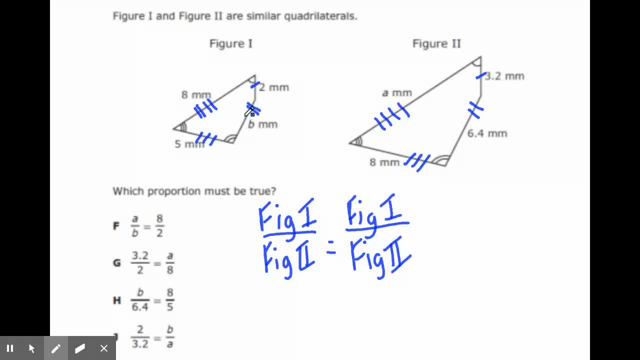 It only has two. All right, so those are not actually corresponding sides And because of that we can't eliminate answer choice F. All right. on G, we have 3.2 and 2.. Those are both corresponding. They are in the same location. 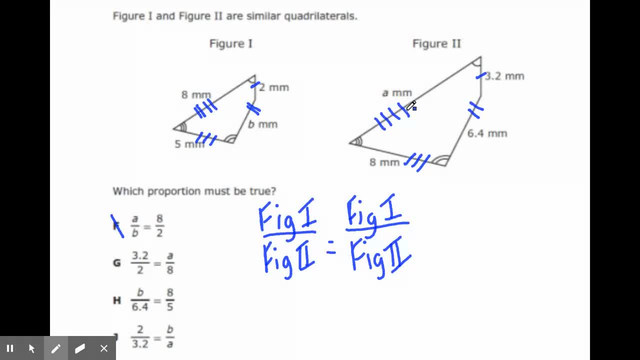 And then we have A over 8. All right, again four and four, So those are corresponding sides. We can see too that figure two is on the left and figure two is on the right, So those are corresponding sides. 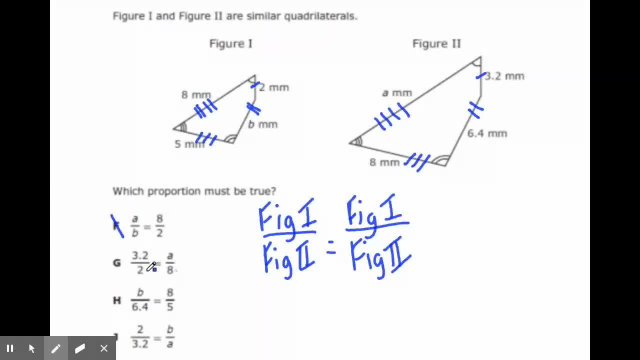 Figure two is on top on the left and figure two is also on top on the right, So that's definitely a contender for our answer. Let's go ahead and mark that, But let's eliminate the other ones, just in case. So H says that B side, B is corresponding. 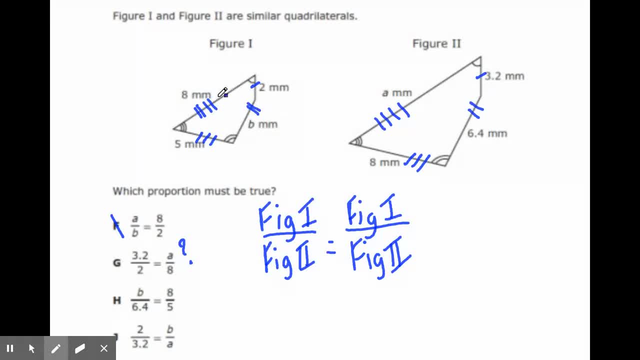 to 6.4, which we can establish is true. They both have two congruency marks and that's over 8 and 5. That equals 8 over 5.. Unfortunately, that's the only thing that's true about our deciding peefer here, because the top three are equ masculine and the top two are greater than positive eyelines. That is the only answer for ourนน marks, But let's just put them all in the bottom row here so you can look around and figure that out for your prawda. 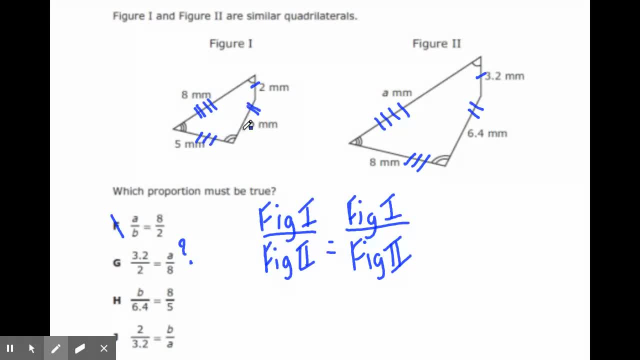 Unfortunately they had figure 1 on top on the left and figure 2 on top on the right, So because of that we can eliminate H. Let's look at J. J says that 2 is corresponding to 3.2.. 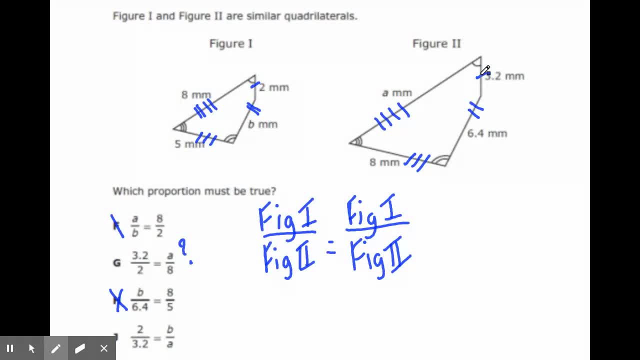 That is true based on our congruency marks, And that equals B over A. All right, so B and A are not corresponding sides. B has two congruency marks and A has four. So because they are not corresponding, we can go ahead and eliminate. answer choice J.